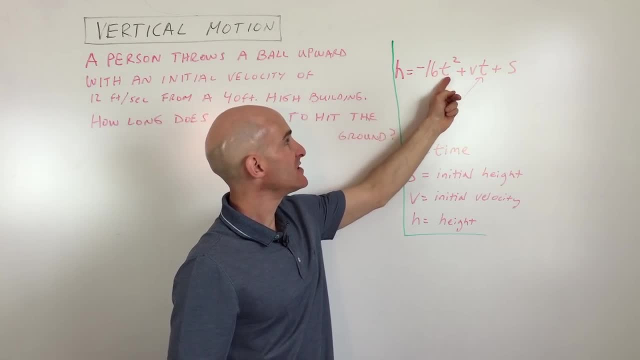 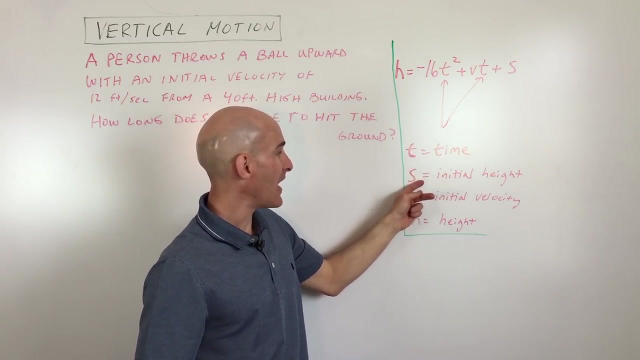 working with is. h equals negative 16t squared plus v times t plus s. So what all those variables represent? Well, the height h is the height right at any given time, t. So t is the time, okay, oftentimes, in seconds, s is the initial height. okay, so that's this here. that's the 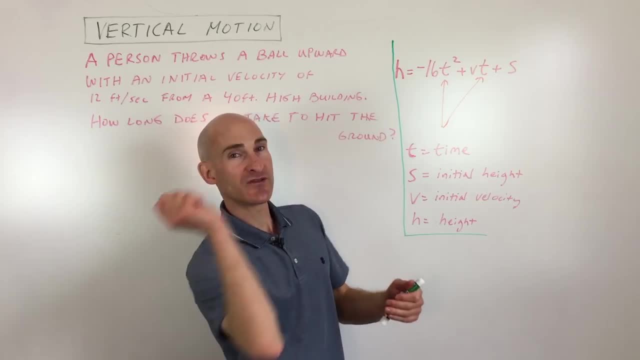 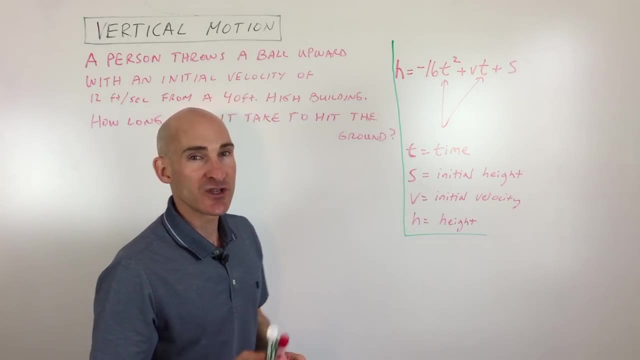 starting height And then v is the initial velocity, so like when it leaves your hand, let's say the item, or when you launch something okay, like an arrow, And then h is the height at any given time. So let's do an example problem and we'll understand this a little bit better. 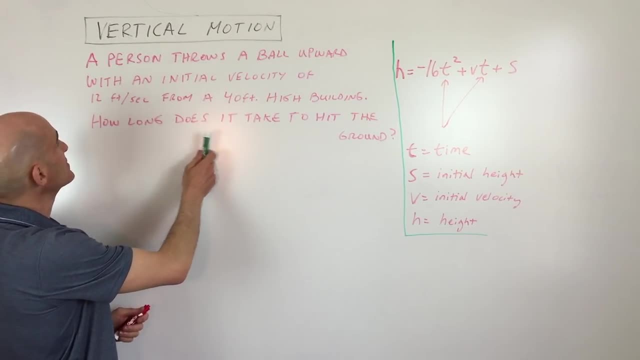 So a person throws a ball upwards with an initial velocity of 12 feet per second from a 40-foot high building. How long does it take for the item to hit the ground? All right, so what we're going to do is we're going to use our vertical motion. 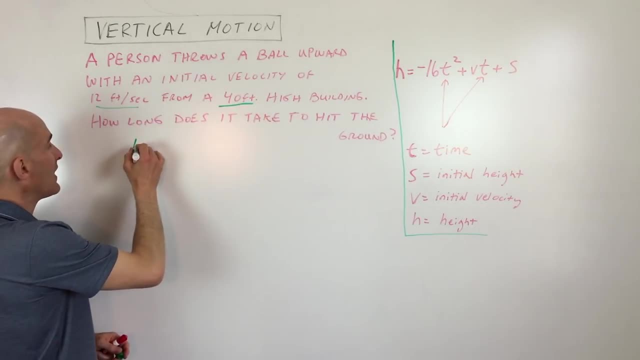 model equation here And what we have is we have h equals negative 16t squared plus v, which is the initial velocity, that's 12 feet per second, so 12t plus the initial height, which is 40.. Okay, so now we have our equation. Now, if you can kind of visualize this, okay, 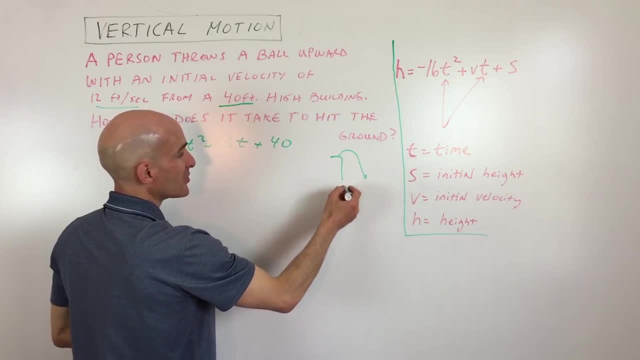 here's the building. The ball is going to look like that and we're trying to figure out where it hits the ground. So we're going to use our vertical motion model equation here. If we want to draw this on an axis, it'll look something like this: Here's time and here's the. 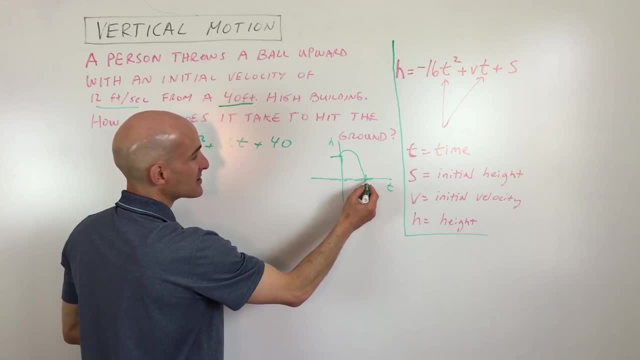 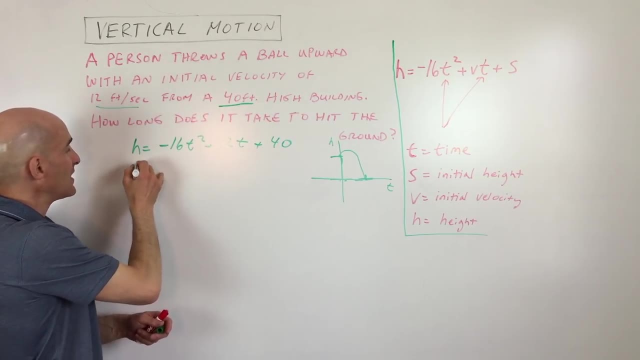 height And basically, what's happening is, as time is passing right, the ball is going up and it's coming back down, and we're looking for where the height is going to be zero. That's where it hits the ground. So let's go ahead and set h equal to zero, And what we can do is we can factor this. 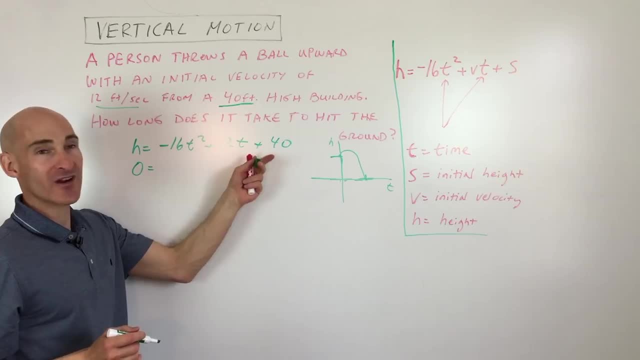 or we could use the quadratic formula, or we could complete the square, or we could graph it on our calculators. We have a lot of different options, but let's see if we can do it, factoring this particular one. So what I'm going to do is I'm going to factor this and I'm going to do this. 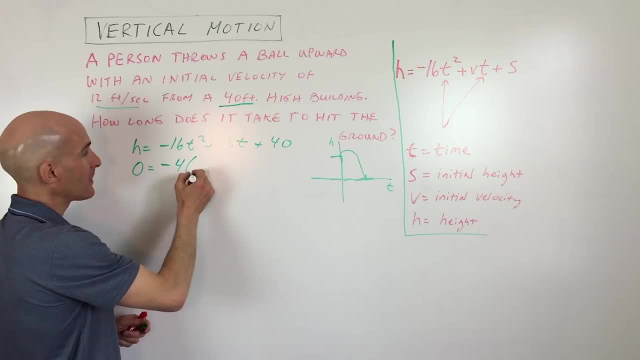 factor out the greatest common factor, which is negative four, So I get four t squared minus three t minus 10.. Okay, And then what we're going to do is we're going to try to see if we can factor this further. So if we take the leading coefficient times the constant, that's negative 40.. What two.